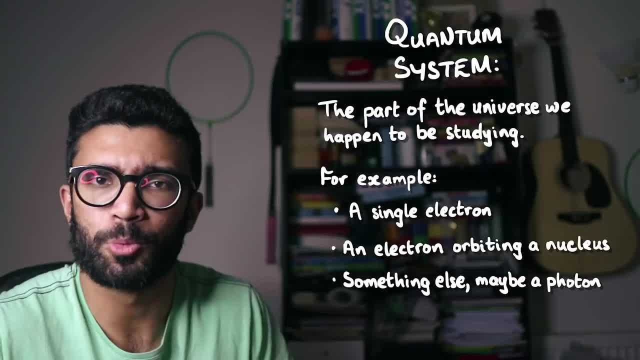 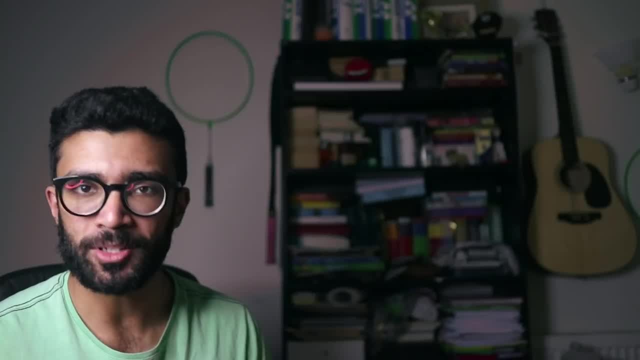 a nucleus, or it could be something else, maybe a photon, whatever. Whatever part of the universe we're thinking about at that point in time is our quantum system, And what makes it specifically a quantum system is that we use the rules of quantum mechanics to analyze this system And the 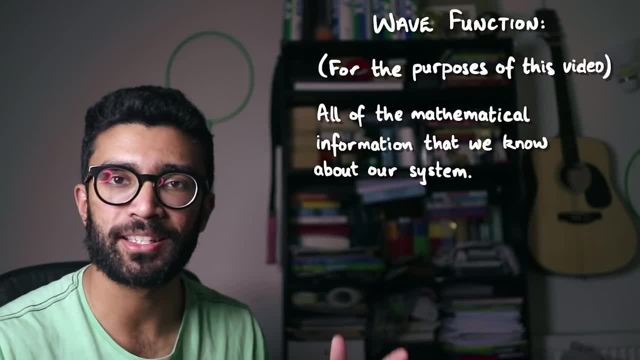 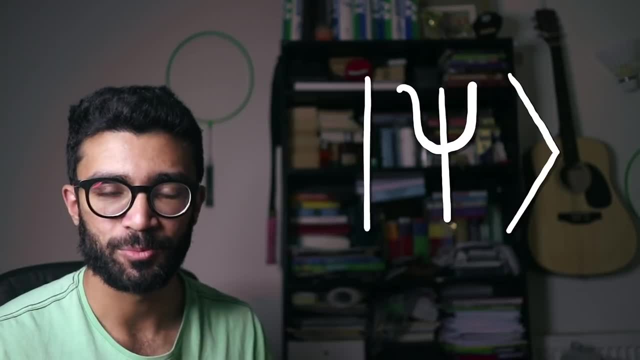 wave function for the purposes of this video is simply all of the mathematical information that we know about that system. But we don't just write psi when we represent a quantum system. We actually write it like this, with a straight line to the left and an angled or pointed bracket, depending. 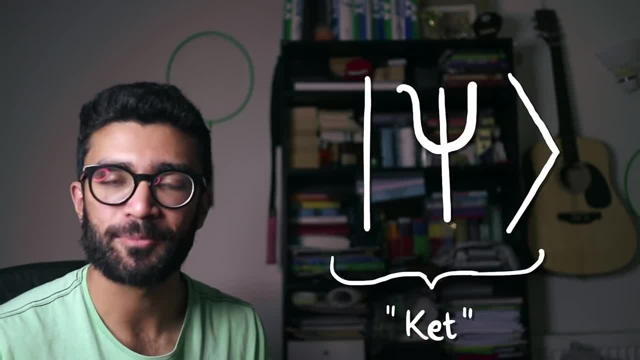 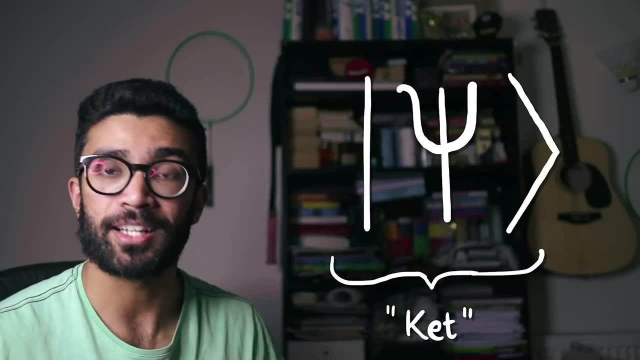 on what you call it to the right. This whole thing is known as a ket. Now we write it like this for many different mathematical reasons, but all we need to know here is that it allows us to differentiate between a ket, a quantum system, and say a constant or some other thing that we'll see. 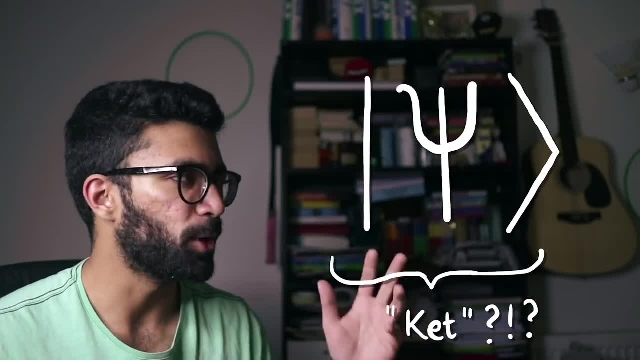 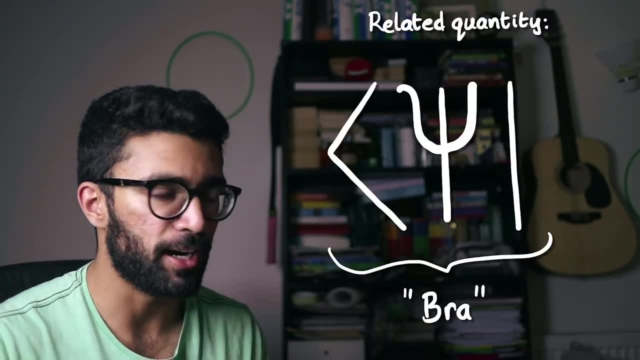 in a future video, known as a ket. So let's get started Now. why is this thing called a ket? Why do we represent the wave function of a quantum system with a ket? Well, because related to a ket is a quantity known as a bra. Why are these things? 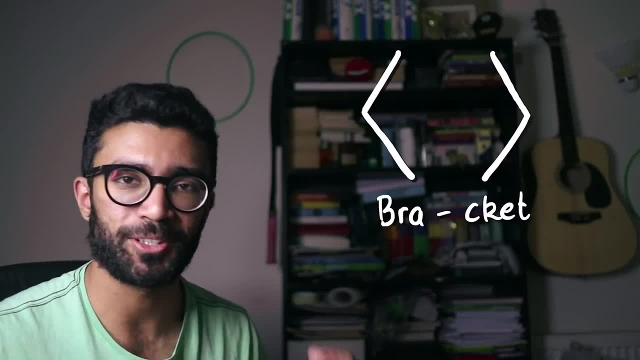 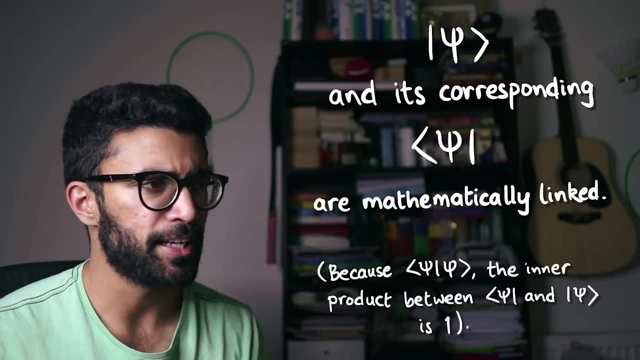 called kets and bras. It's because it comes from the word bracket. We've got the bra here and you've got the ket here. Now, a ket and its corresponding bra are mathematically linked in a very fundamental way. In other words, if we talk about the ket psi, which is used to represent the 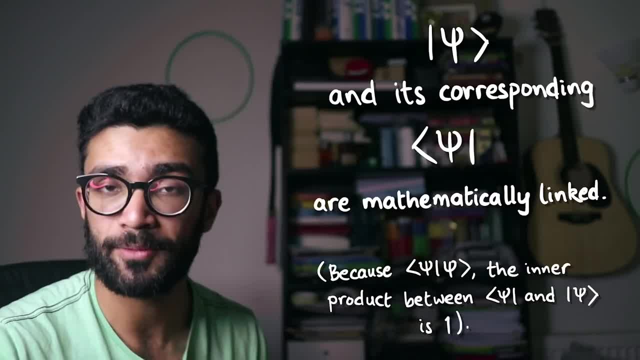 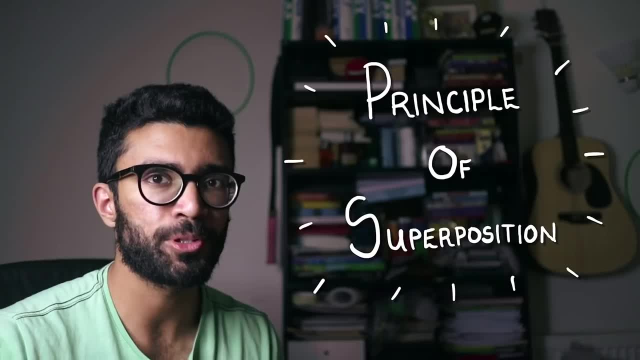 wave function of our quantum system and we look at the bra psi. then the bra psi and the ket psi are linked mathematically, Anyway. now here's the thing Many of you may have heard of the principle of superposition being an important thing to quantum mechanics. You may just have 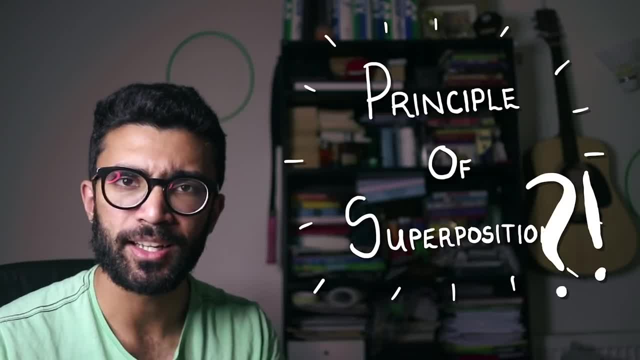 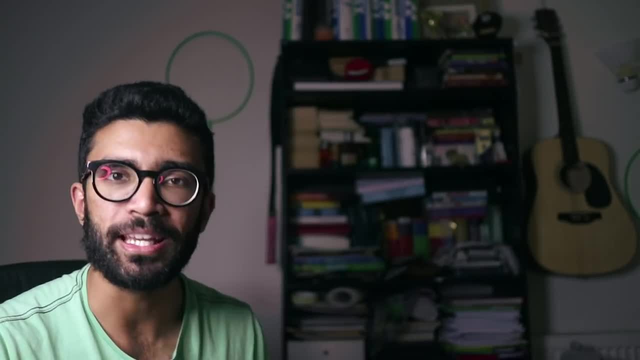 not heard it being called the principle of superposition. The idea is that when our quantum system is left alone, it is in a blend, a soup of all possible states that it could be in, For example, if our quantum system simply consists of an electron and we are thinking about 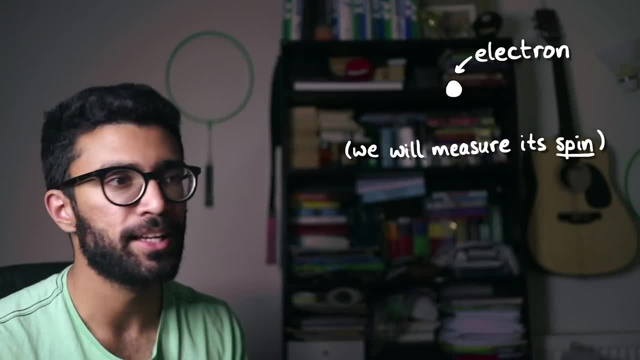 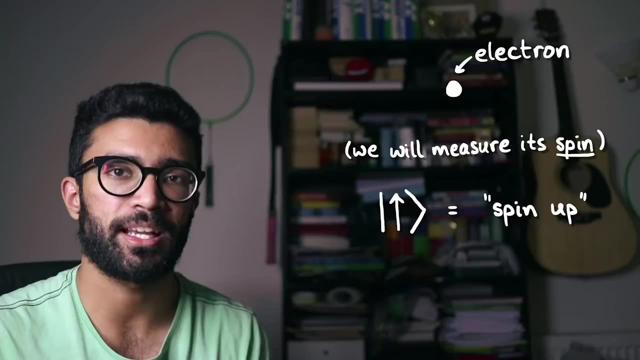 measuring its spin. say its spin is a property that this electron has. this electron could be found in one of two possible spins. It could be in a state known as spin up and it could be in a state known as spin down. We don't really need to know exactly. 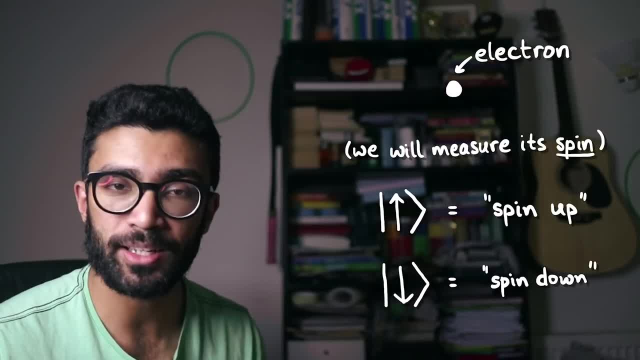 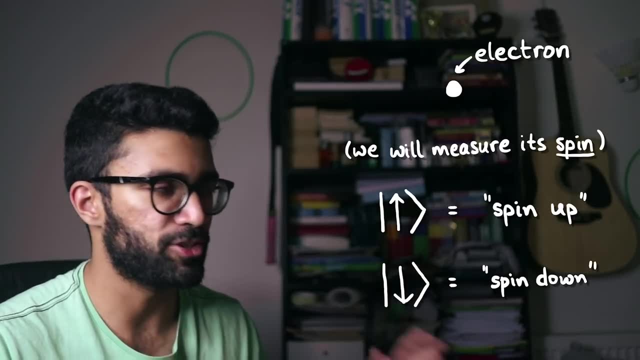 what these mean. but all we need to know is that there are two possible states that we could find our electron in if we were to go and measure its spin. Now here's the thing: If our electron, our quantum system, is just left alone, then it is said to be in a superposition of both of these. 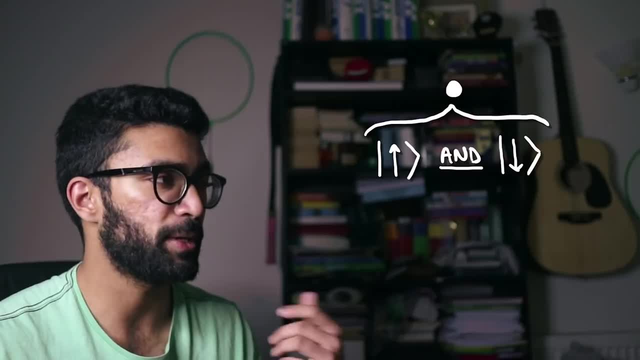 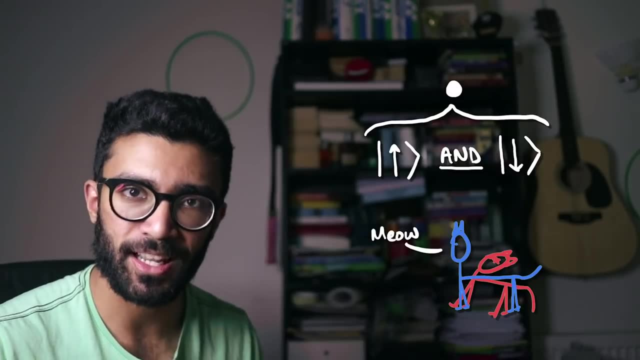 states. In other words, many people like to think of it as spin up and spin down at the same time, or, you know, an equivalent way of thinking about it is Schrodinger's cat being dead and alive at the same time, which in itself brings up a lot of problems, but we're not going to address them. 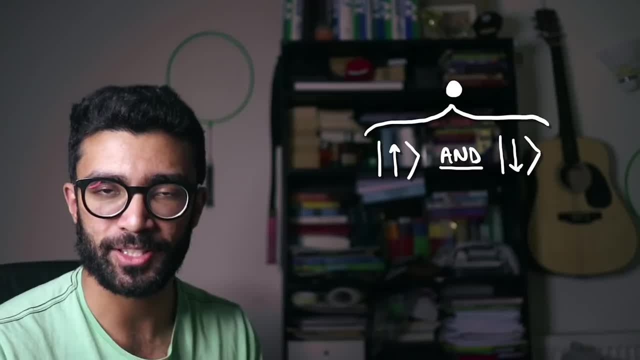 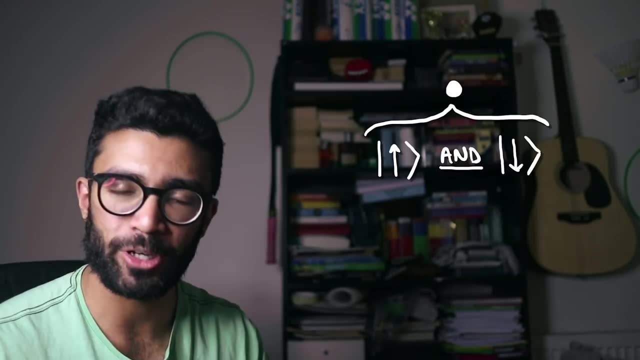 here. All we need to know is that our quantum system can be in a superposition of states. It can be in, supposedly, more than one state at one time, but that's only if it's left alone and nothing is interacting with it, and we're not making any measurements or anything like that. 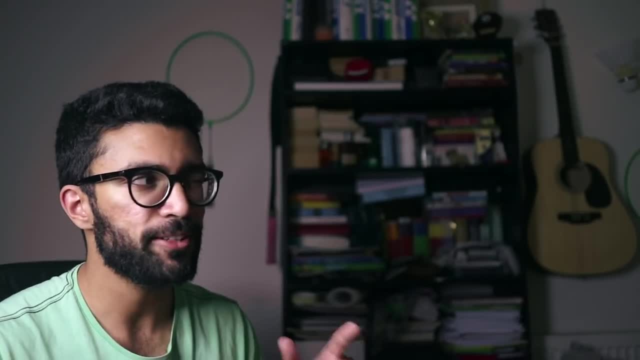 By the way, if you want to hear a slightly deeper discussion about spin, I haven't yet made a video about spin specifically, but I have talked about spin in my previous video on quantum entanglement. Go check that out if you haven't already. So if you're interested in learning more about spin. 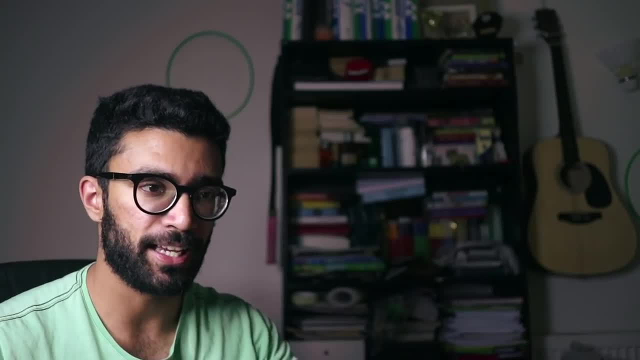 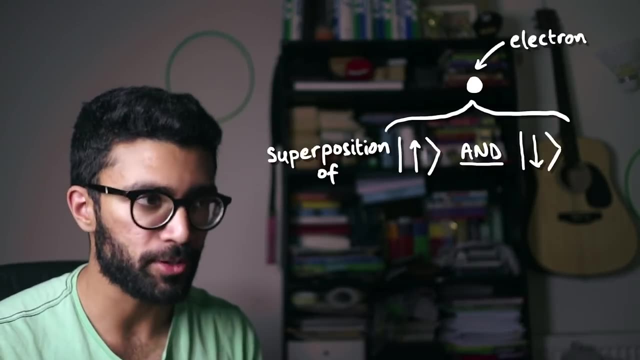 I discuss what quantum entanglement is and try and explain the concepts you need to know about quantum entanglement. For now, though, all we need to know is that our electron can be in either the spin up state or the spin down state when we measure it, and when we've left it alone, it's. 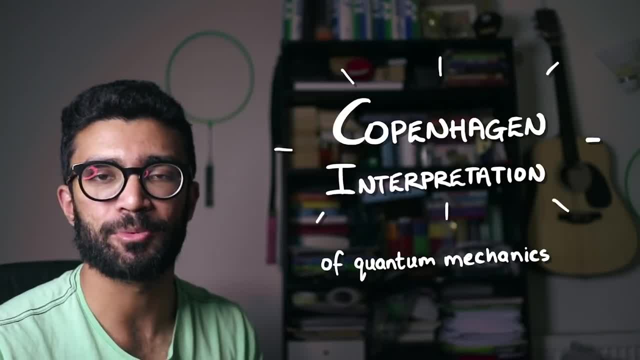 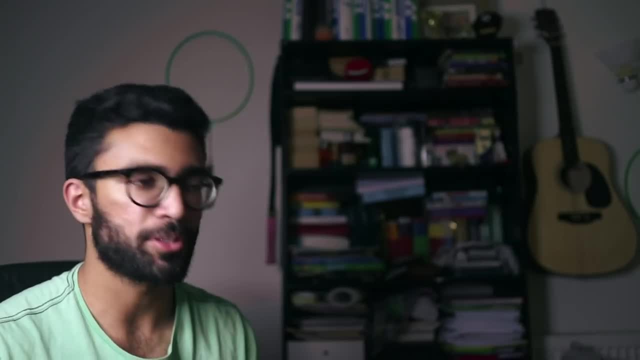 in a superposition of the two states. At least that's what the Copenhagen interpretation of quantum mechanics tells us, which is by far the most common interpretation of quantum mechanics at the moment. Now, in a situation where our quantum system, in this case an electron, 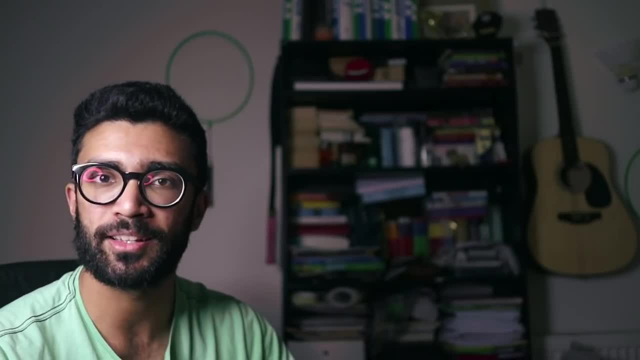 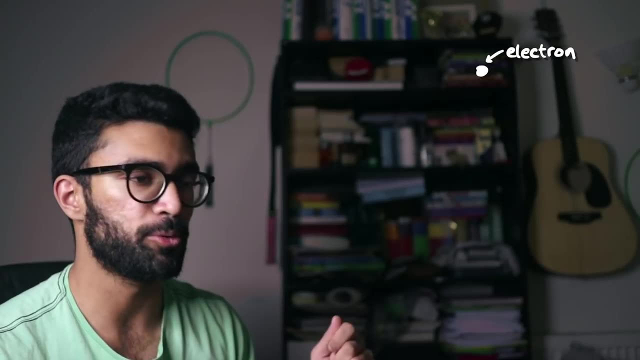 is just being left alone. nothing is being done to it. it's not interacting. it's not interacting with anything and we're not making any measurements on it. we can write the wave function of our electron as a superposition of the two possible states that it could be in. 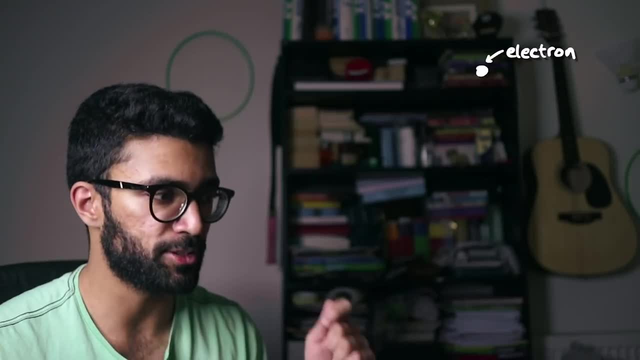 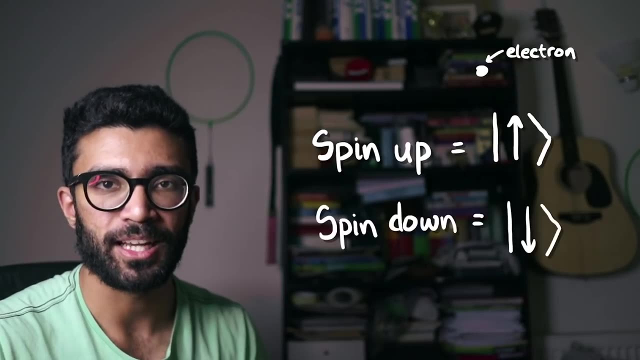 spin up and spin down, And the way that we can do that is to add the two states together. So we can write our spin up state like this and we can write our spin down state like this, And when we add them together with numbers in front of each state, we'll come back to those in a second. 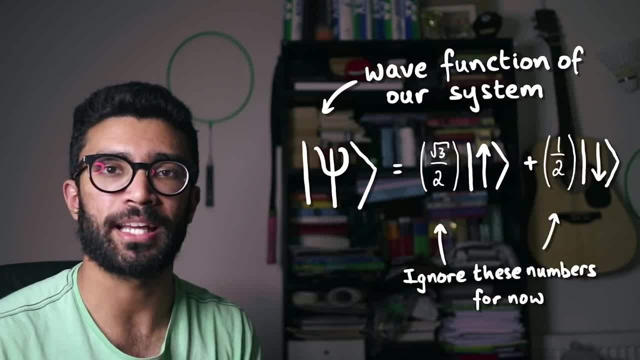 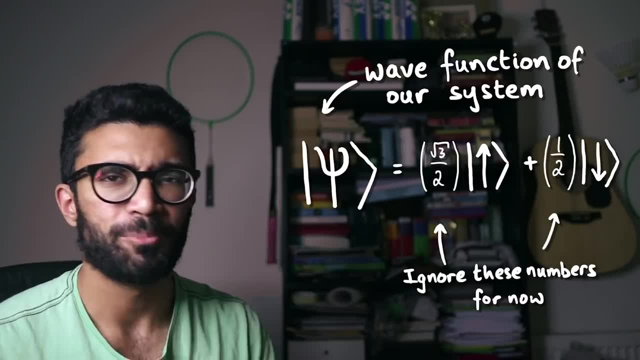 essentially, what we're doing is giving a representation of the overall state of our system, the overall quantum state of our system. It's in a superposition, a sort of blend of both spin up and spin down. But here's the thing: when we actually go and measure the spin, 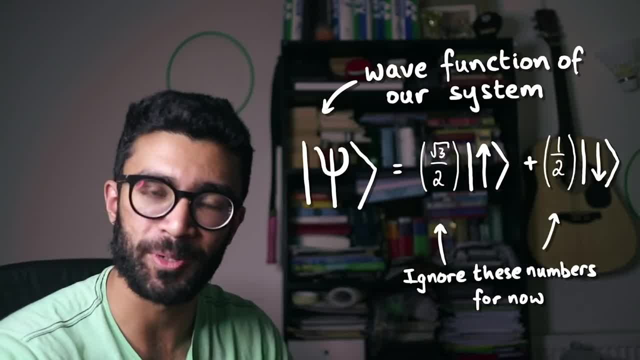 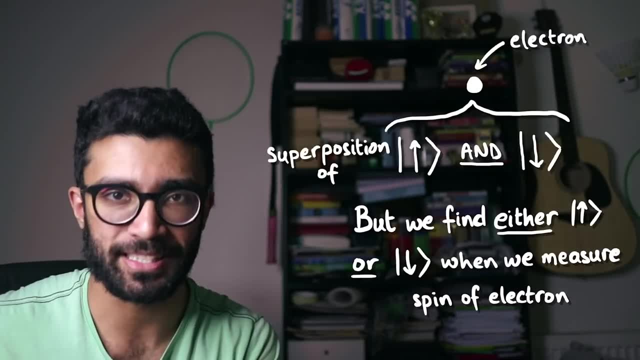 of this electron. let's just imagine that's a thing that we can do without worrying how we do it. when we go and measure the spin of this electron, we will only ever find it to either be in the spin up state or the spin down state. What happens is our wave function, which initially was a. 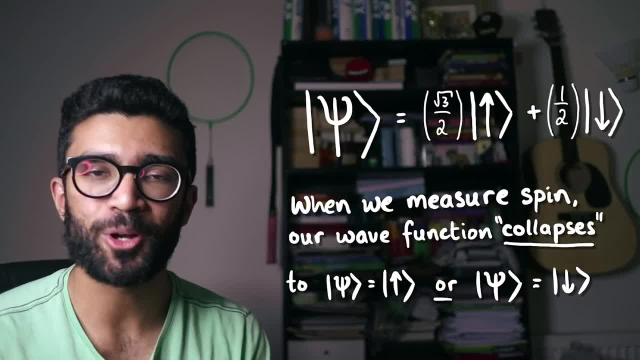 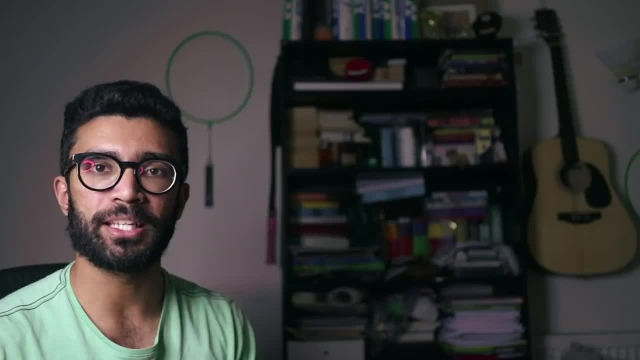 superposition of the two states collapses into just one. This phenomenon is known as the collapse of the wave function. Pretty creative, isn't it? So if we go and measure the spin of this electron- this is the important thing, though- we will never find our system to be in a superposition of both. 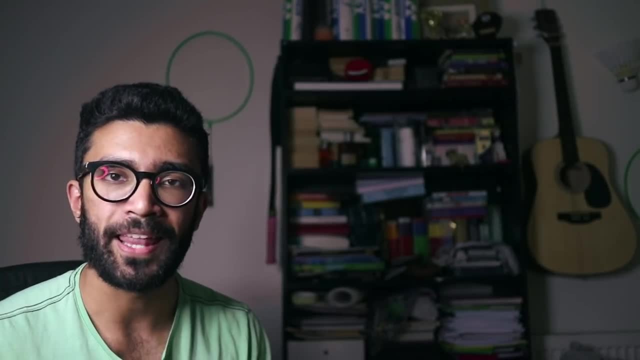 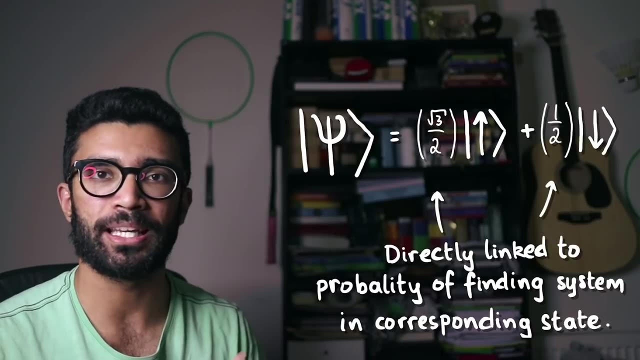 states. when we measure it, we will only find it to be in one or the other, And this is where the numbers in front of each state come in. The numbers are directly linked to the probability of us finding the electron to be in a particular spin state, In other words, the number that is in front. 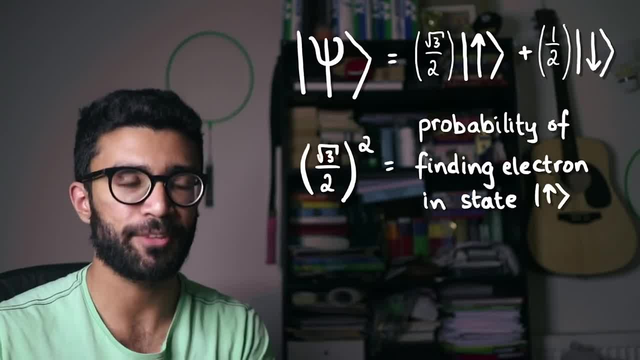 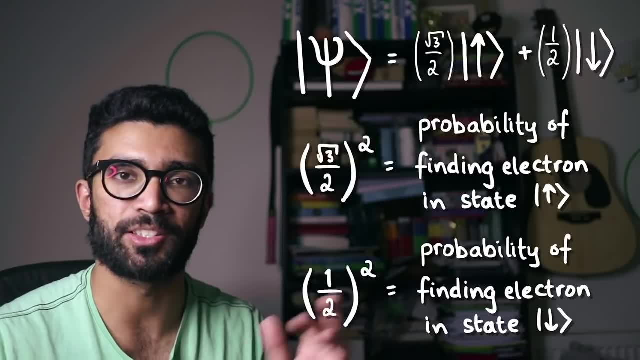 of the spin up state. when we take that number and we square it, that gives us the probability of us finding the particle in the spin up state And equivalently with the spin down state, if we take the number in front of the spin down state and square it, we get the probability of us finding the 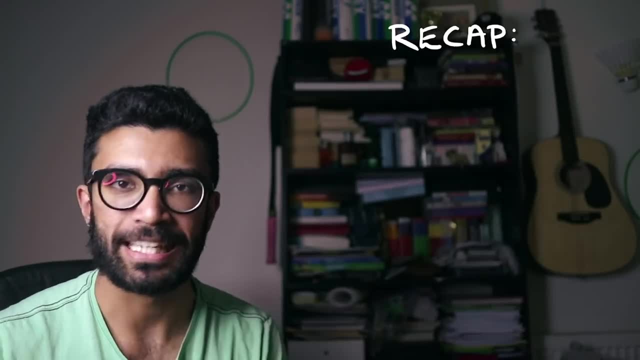 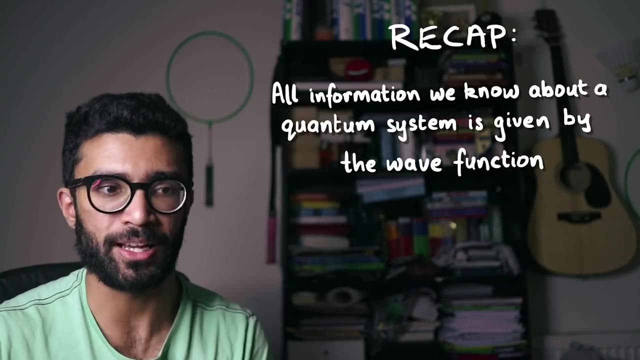 electron in the spin down state. And now let's quickly pause and think about how far we've come from the beginning of this video. We now understand that a quantum system can be represented by what's known as a wave function, the wave function being all the mathematical information we have about a 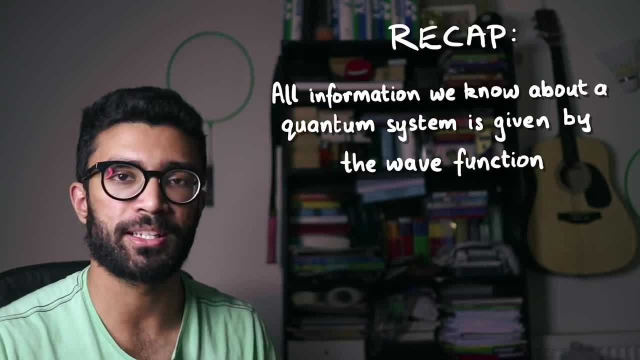 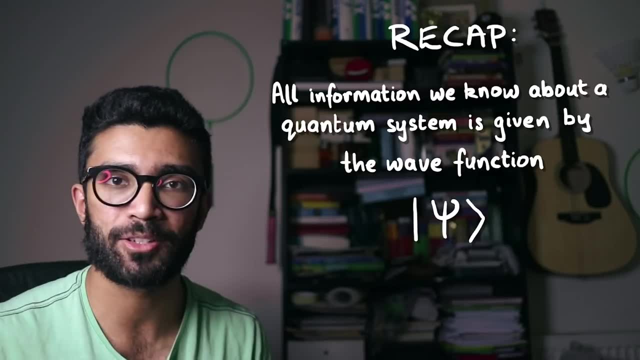 system and we know that that wave function can be often represented by the Greek letter psi. but we don't just write it as the Greek letter psi. we also have a line on the left and an angle bracket pointing to the right. on the right of the psi. This represents what's known as a ket and that 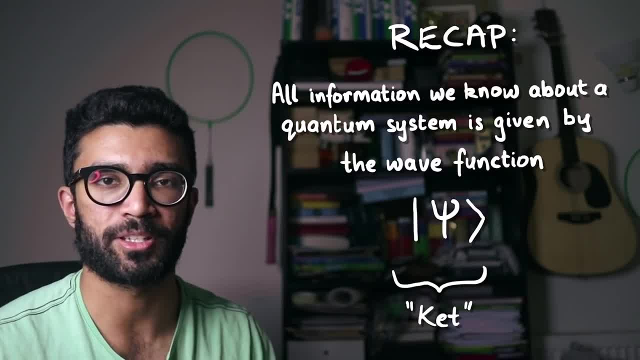 ket is just a mathematical way of saying that a quantum system can be represented by a wave function. It's a way of representing all the information that we know about our quantum system. Additionally, we also have realized that quantum systems can be in superpositions of possible measurement states. 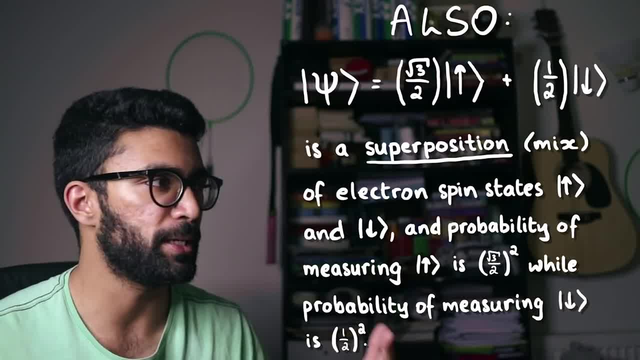 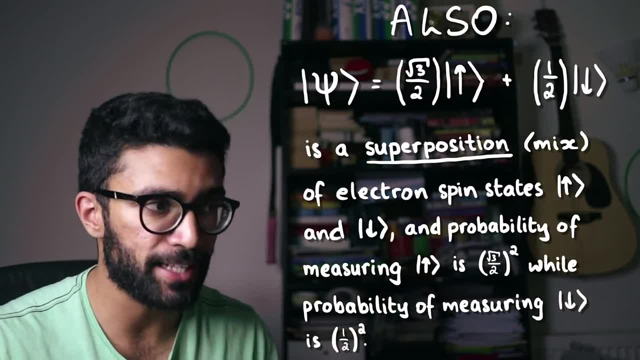 which essentially means that when we go and measure our system, we can find our system in any of these states, but while we're not measuring it and while nothing is being done to the system, it is in a superposition or a sort of blend of all possible states. Additionally, we've seen that the 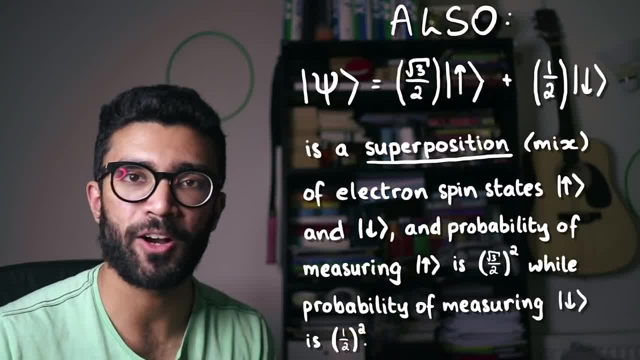 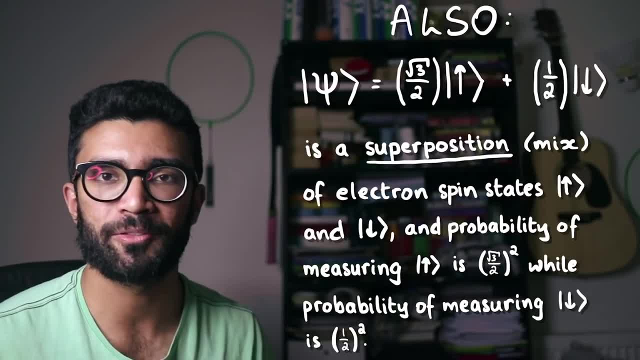 numbers in front of each state are directly linked to the probability of us finding our system in that state when we measure it. So already we're learning the language of quantum physics. We are realizing how quantum physicists write quantum states. Now there are a couple of points I want to make about what we've learned so far. Firstly, this is all why. 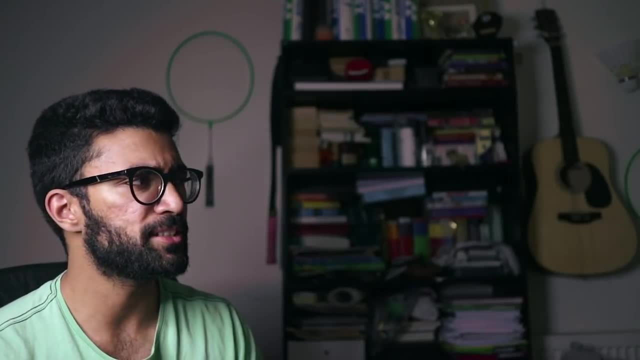 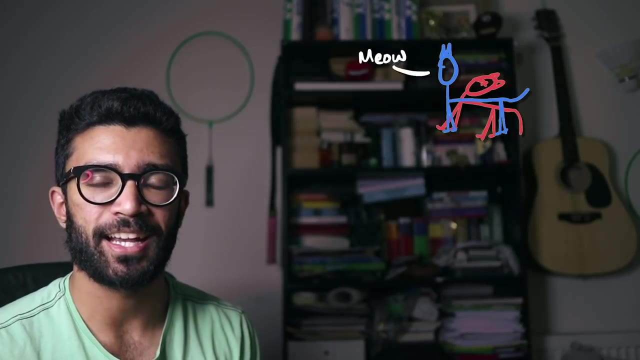 quantum physics is so extremely weird, The idea that a quantum system can be in a mixture of all possible states. that's like saying: you know, on a macroscopic scale, on a large scale, Schrödinger's cat is dead and alive at the same time. Again, that doesn't happen. We're not going to talk about that. too much. Or even like on a macroscopic scale a switch is both on and off at the same time- Again, really weird, and macroscopic analogies don't work that well, But when scientists realize that there's a possibility this might happen on the small scale, that's what freaked them out, You know. 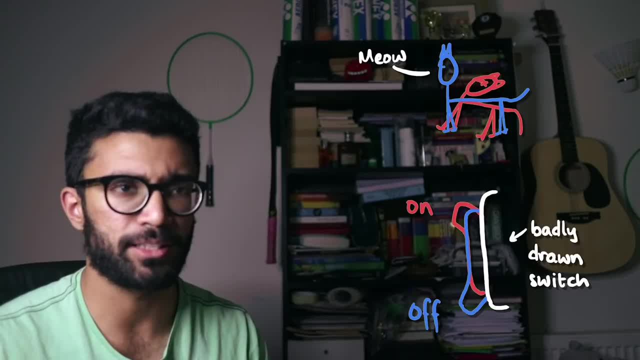 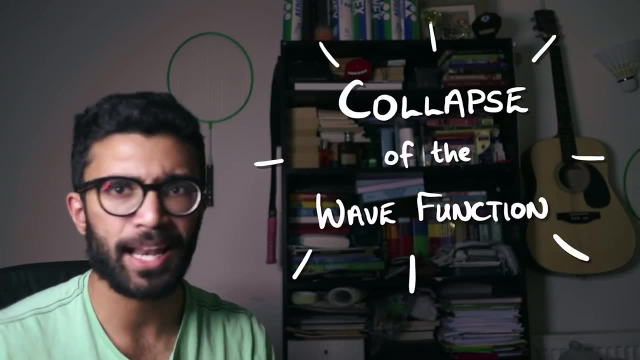 it's a really strange concept that a system can be in two states at once. The other thing is that when we measure our system, it's still only ever going to be in one possible state. The whole collapse of the wave function thing is really weird. The fact is that we will never find it to. 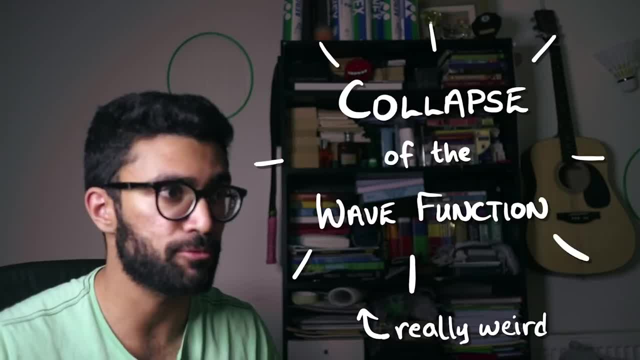 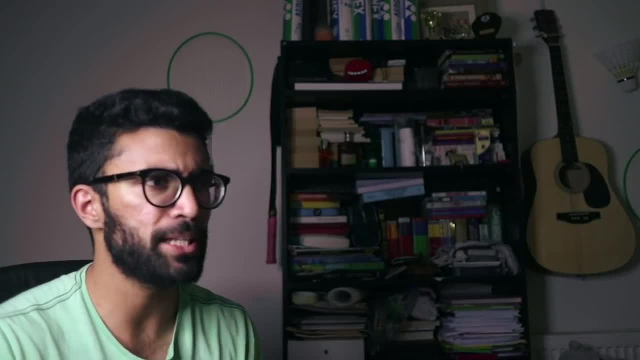 be in a superposition of all states, but there are other effects that allow us to realize that our system is in a superposition, And yet the idea that making a measurement yields a probabilistic result is also extremely weird. Interestingly, we cannot predict what the result of a particular 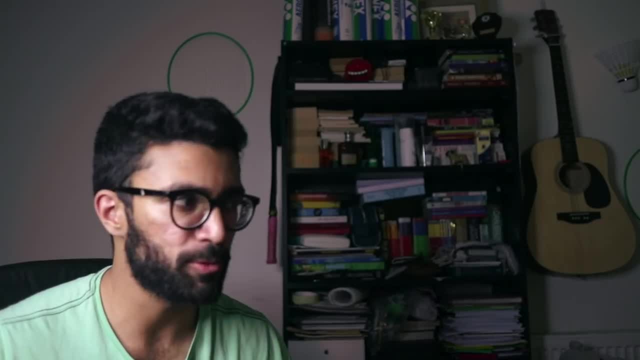 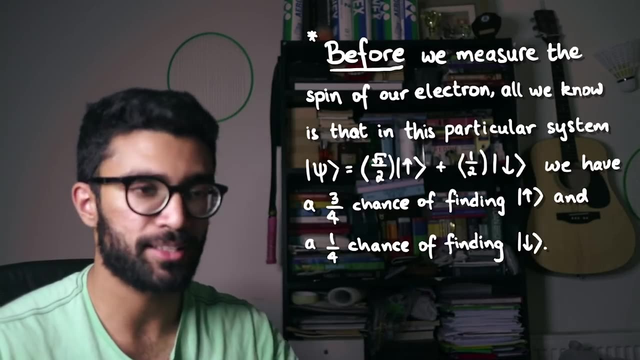 experiment is going to be, We can only predict the probability with which we will find a certain state. So when we, when we measure the spin of our electron, all we know is that in this particular system, we have a three quarters chance of finding it in the spin up state and a one quarter chance. 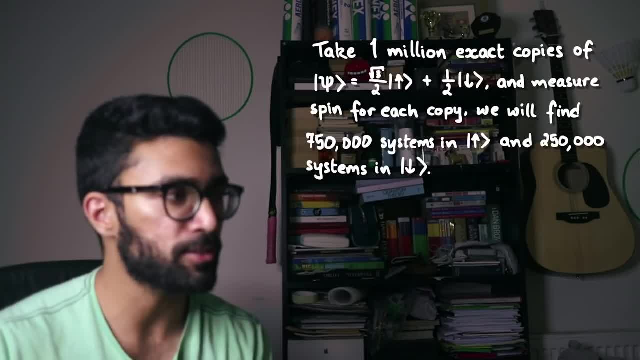 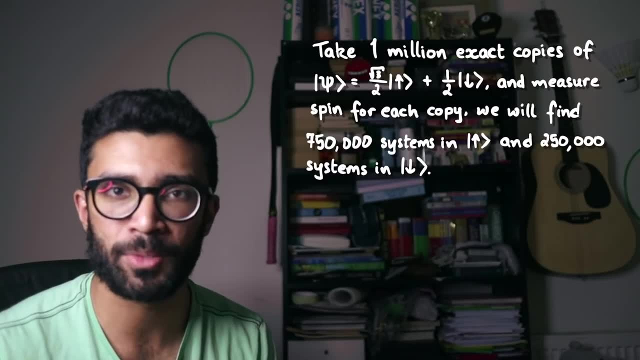 of finding it in the spin down state. This is equivalent to saying that if we took lots and lots of exact copies of our system- so let's say we had one million exact electrons like this set up in exactly the same system- then three quarters of a million of those electrons will be found in the 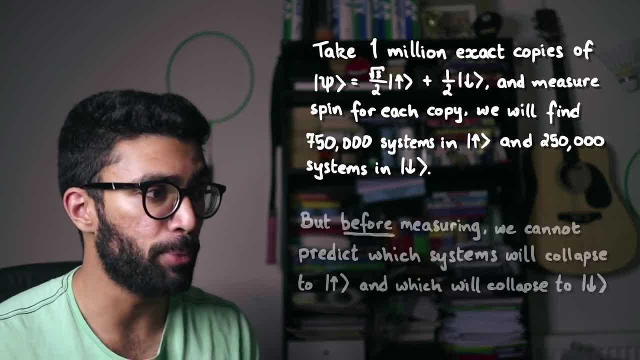 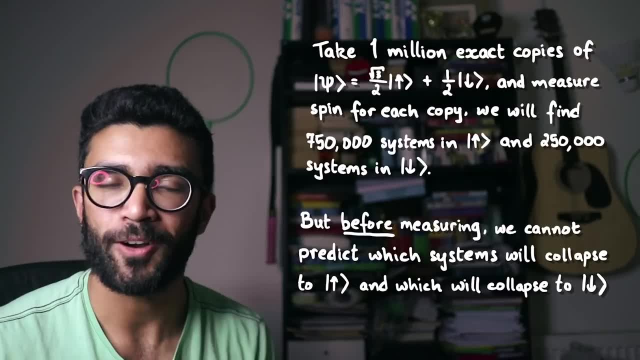 spin up state and one quarter of a million will be found in the spin down state. But we cannot ever, before an experiment, go and say that this one is going to be in a spin up state and this one is going to be in a spin down state. Finally, one more way to look at this whole thing, if your mind hasn't. 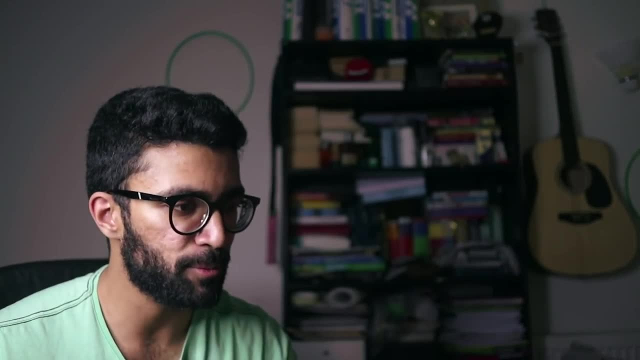 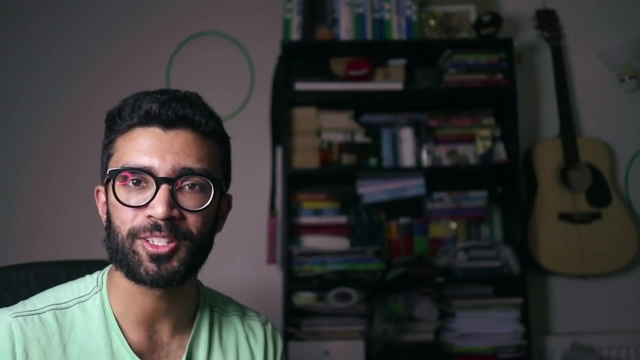 already been boggled. If we take our system and set it up exactly the same way once again and take it exactly the same way, we might get a different result. This is something that I want to talk more about in future videos, so if you want to see more of that, then let me know in the comments down. 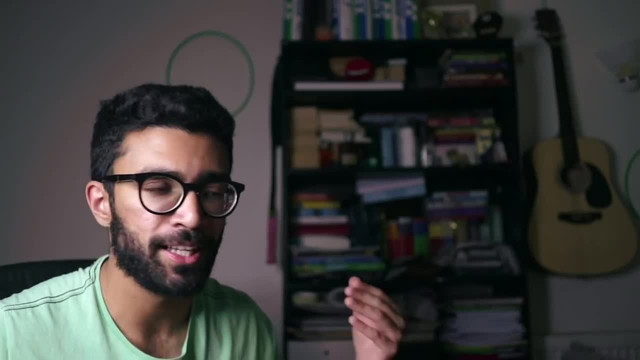 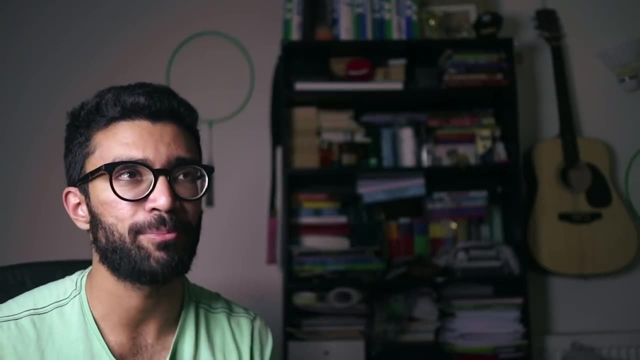 below, But this is the stuff that really interests me when it comes to quantum information. This is kind of the stuff that I enjoyed most when I was studying at university, and this is the kind of stuff I like making videos about. However, don't worry, I am actually planning a few special 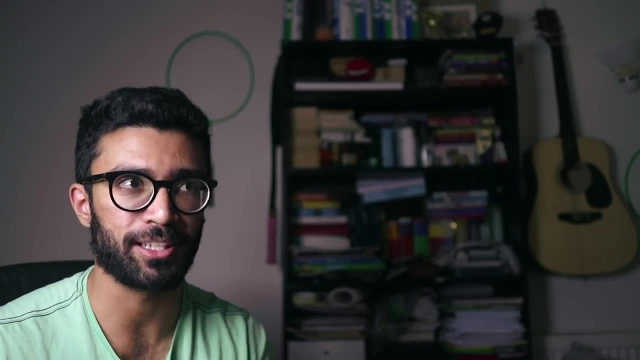 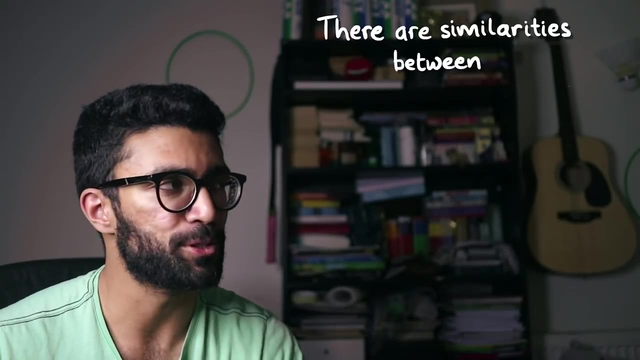 relativity and general relativity videos. so stick around for those if you're interested in more of the relativistic stuff. Anyway, let's get back to what we were talking about Now. here is where it gets really interesting. There are a lot of mathematical similarities. 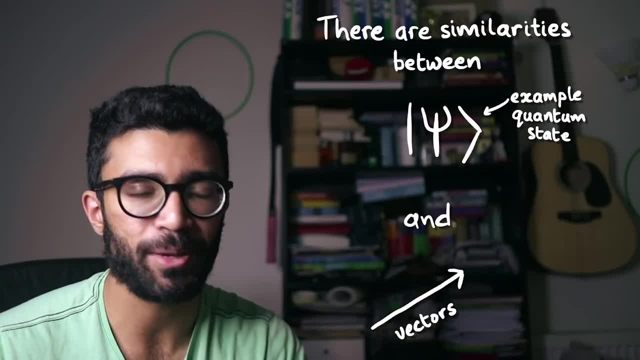 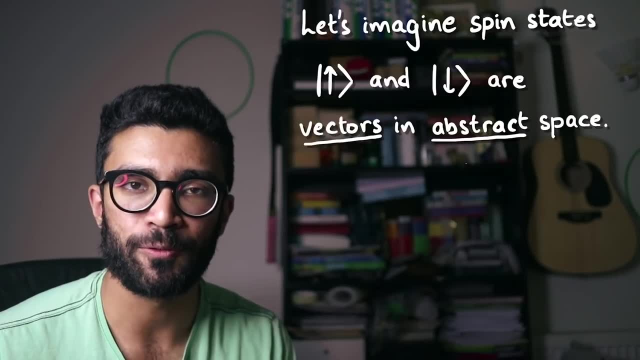 between quantum states and vectors. In fact, there's a really neat mathematical way of describing quantum states as vectors For any given quantum system. each particular state that our system could fall into when we make a measurement on it can be thought of as a vector. in 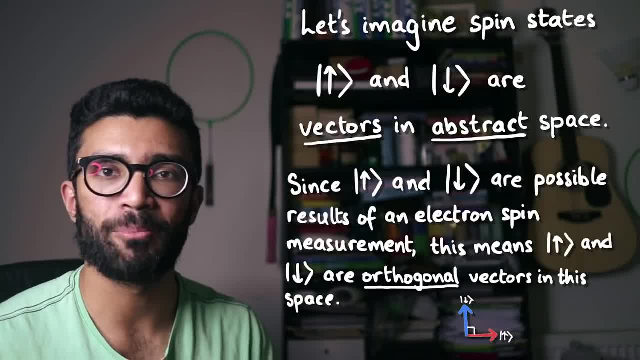 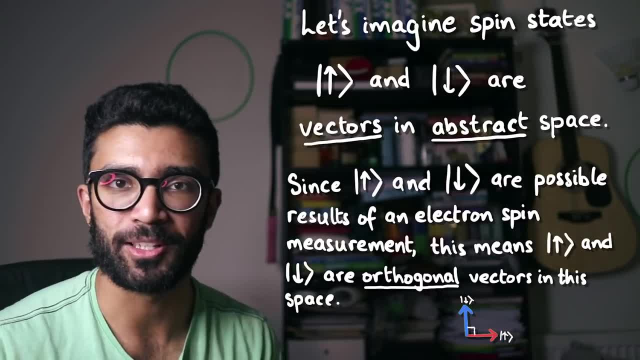 some abstract space. Importantly, each possible result of our measurement is a vector that is orthogonal to every other result of our measurement. Orthogonal means at right angles too, by the way. So coming back to our system, which is just an electron, the two possible results we 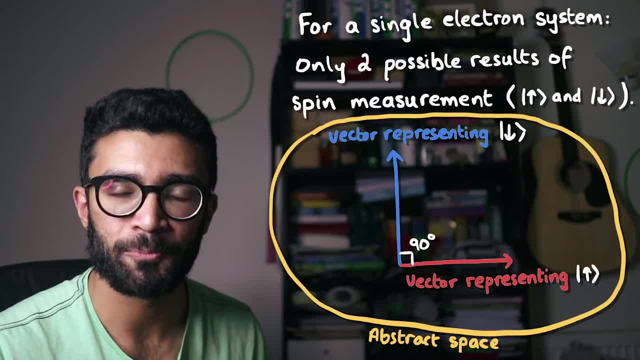 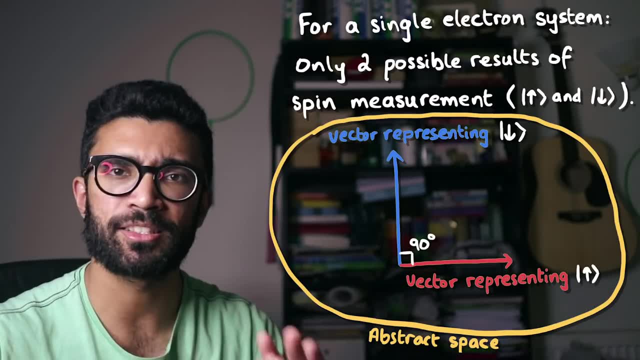 could find when we measure its spin, are spin up and spin down. Now, spin up and spin down can be each represented by a vector and the spin up vector in this abstract space. this is not real space, this is just some mathematical space can be thought of as being mathematically orthogonal. 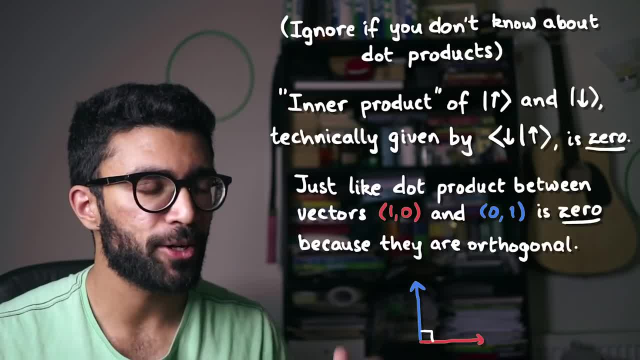 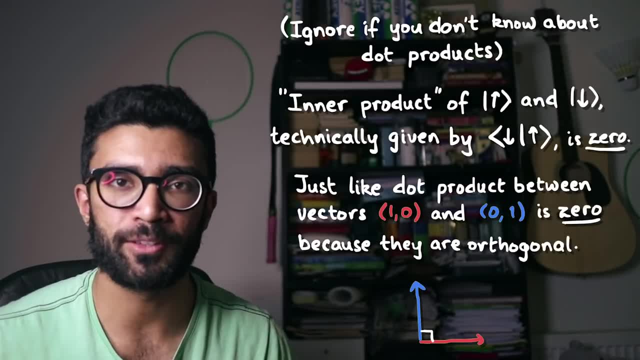 or at right angles to the spin down vector. Now the reason that we know that these vectors are orthogonal to each other is, if you know about dot products between vectors, the dot product or the mathematical equivalent for quantum states of two of these vectors. any two of these possible. 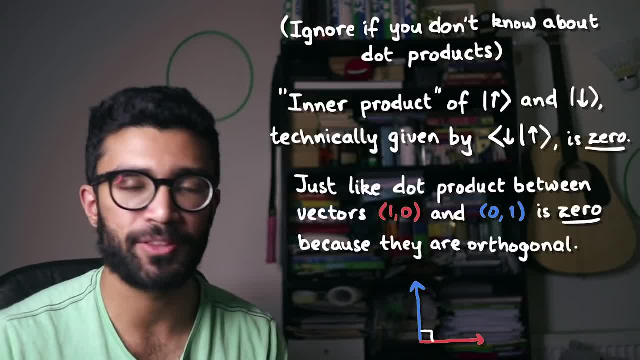 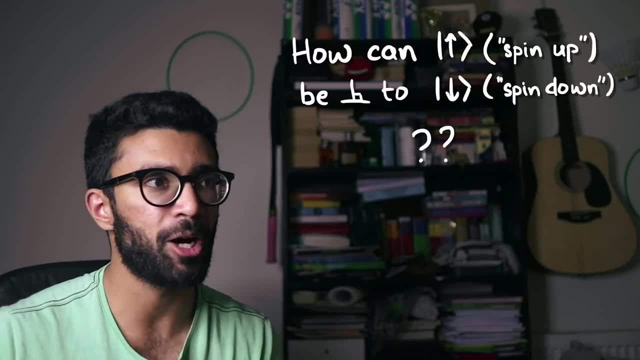 results is zero, Which means that they behave as if they are two vectors that are orthogonal to each other. Now, this might seem a bit strange. How can spin up be orthogonal to spin down? How can up be pointing at 90 degrees to down? Well, remember, like I said earlier, this is just some abstract. 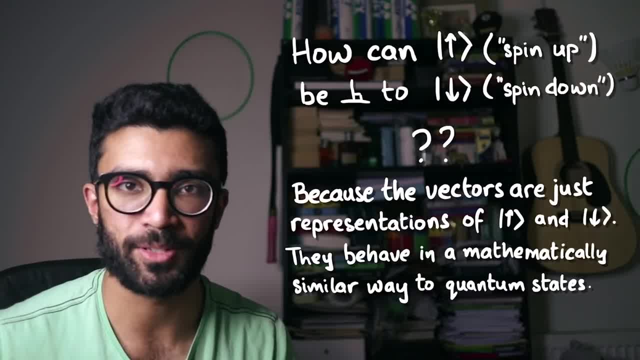 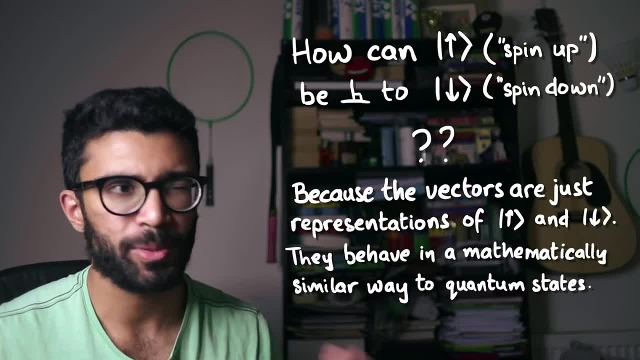 mathematical space that allows us to represent these quantum states in such a way that they behave like vectors. Additionally, we're not trying to say that up is at right angles to down. Spin up and spin down are just names for our quantum states. If you want to know more about these, 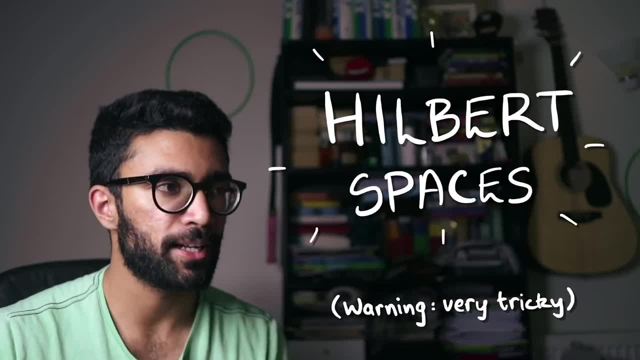 abstract spaces. you can go to the link in the description below. If you want to know more about these abstract spaces, then look up Hilbert spaces. So now, because we've realised that spin up and spin down are two possibilities of a measurement on our quantum system, this means that they must 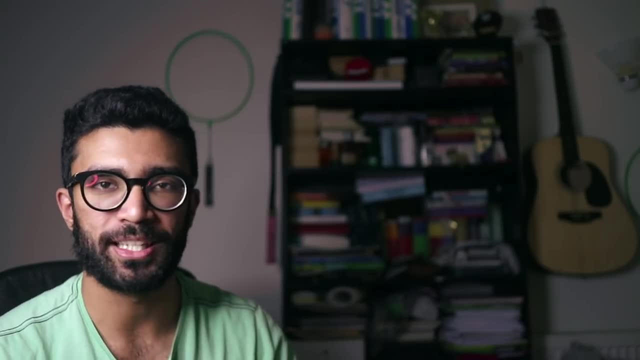 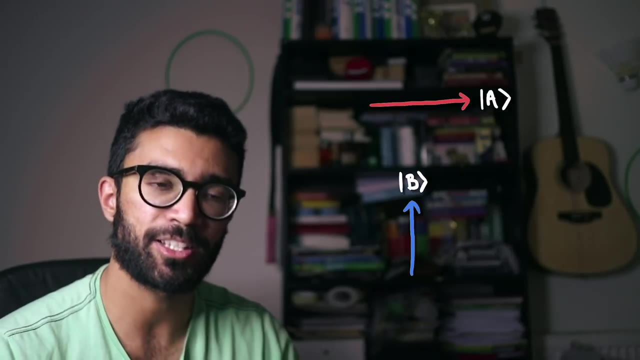 be orthogonal to each other. So let's just represent spin up as pointing in this direction and spin down as pointing in this direction. If that's too confusing, we can call it something else. Why don't we just call it spin state A and spin state B? Because, once again, up and down are. 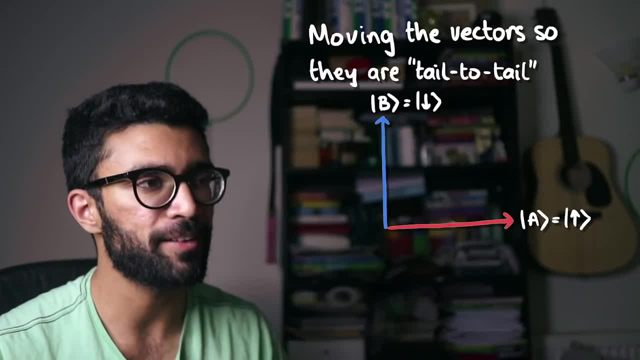 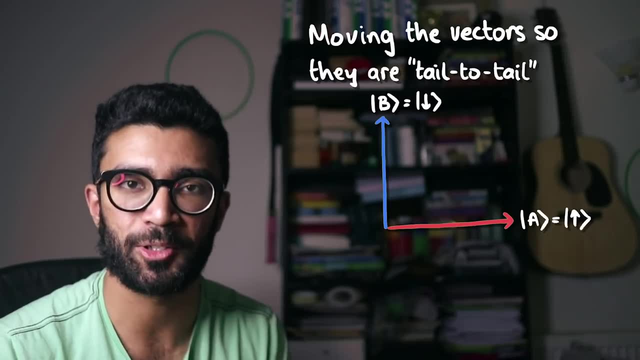 just labels. We don't really need to know what those labels are. What we care about now is that we've got two possible results of the measurement, and these two possible results can be represented as vectors, and these two vectors are orthogonal to each other. So why are we actually going to all? 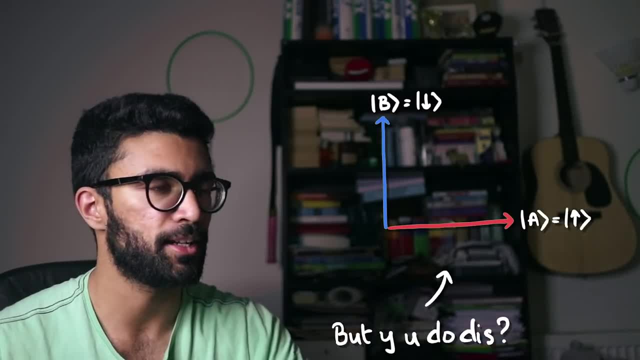 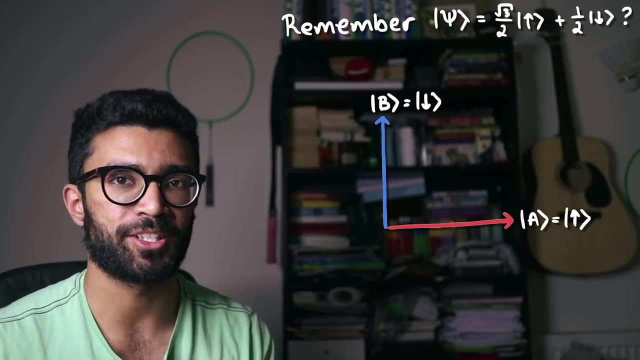 the trouble to do this. Why are we representing our quantum states as vectors? What's the point? Well, the point is: remember the state of our quantum system before we measured it. Remember how it was. in a superposition of states, We can represent our quantum state. 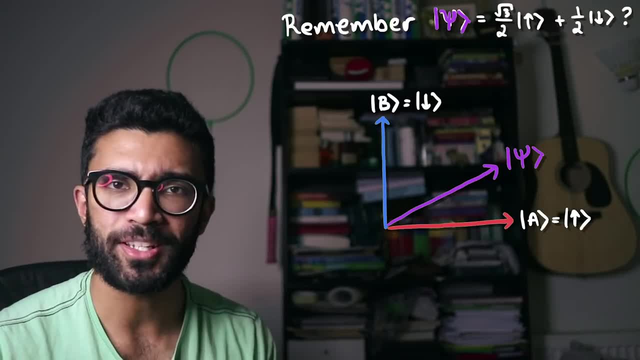 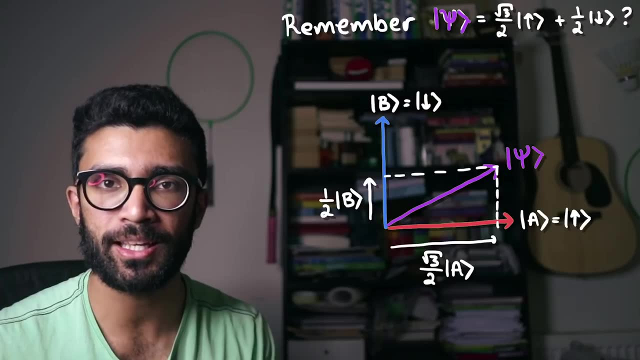 our superposition of states. as just one arrow on this abstract vector space, We can think of our two individual measurement vectors- spin up and spin down, or spin state A and spin state B- as vectors pointing in the x direction and the y direction. These will be our x and y axes on a grid. 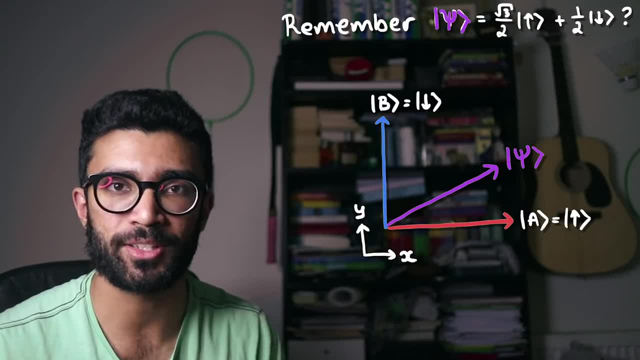 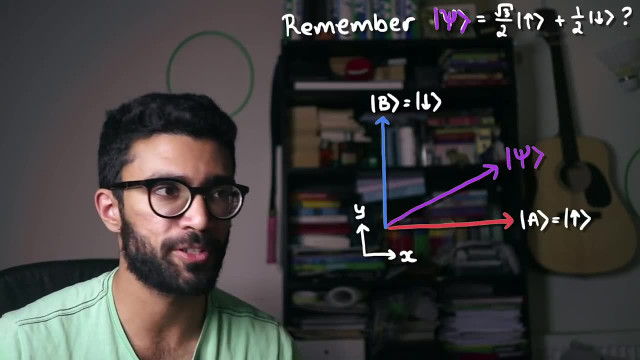 And we can represent any system that is in a superposition of these two states on this diagram that we've drawn, Because remember our initial quantum state, before we measured it was a superposition of some amount of spin up and some amount of spin down. 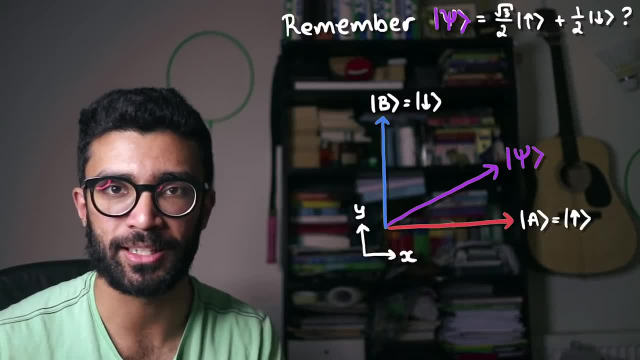 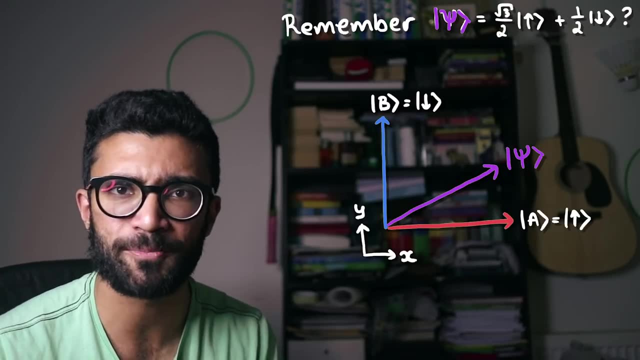 which means that it's some amount of spin up plus some amount of spin down. And when we add vectors together, we just create a new vector in this space, in this abstract mathematical Hilbert space. So we can represent our quantum system before we measured it as this vector here And after we measured it. let's say we found it to be in the spin up state, it collapses to the x-axis in this particular case, the way we've drawn the diagram. So our quantum system upon measurement collapses from this angled vector straight to this vector here. Equally, if we found it to be in the spin down state, it would: 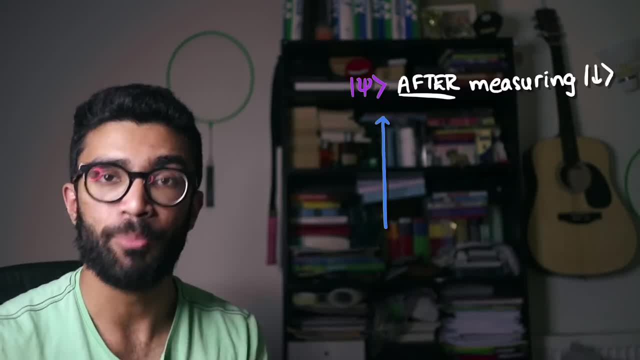 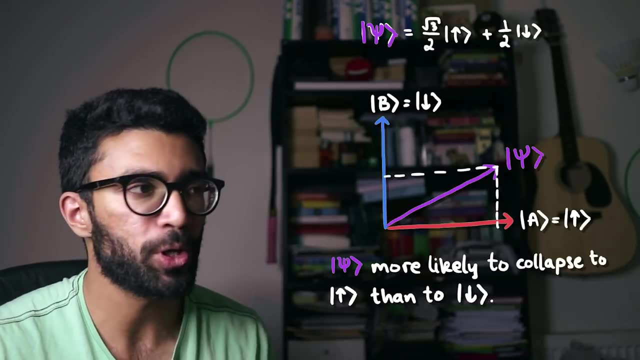 collapse from its initial position to the other axis. But we can also see that, because our initial measurement is added to slightly less spin down, it's more likely to snap to the x-axis in this particular case than it is to the y-axis and therefore we're more likely to find a result of 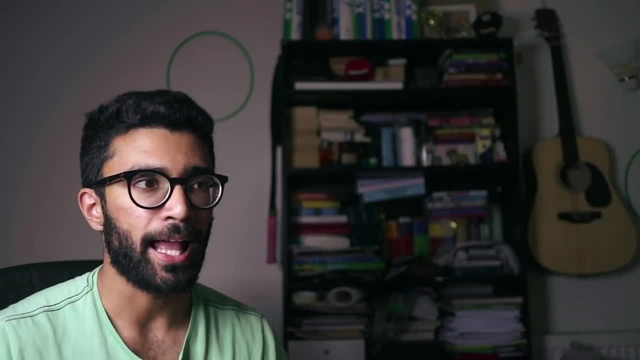 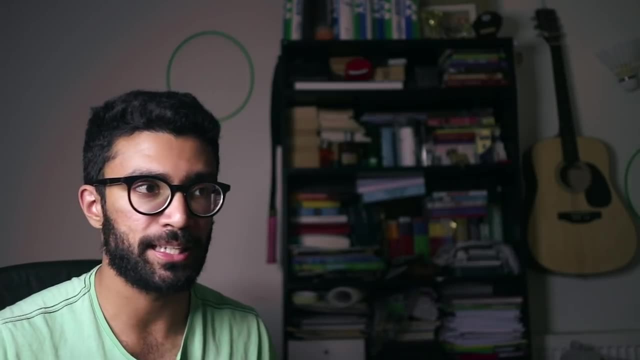 spin up. So this is where representing quantum states as vectors comes in handy. Any possible result of a measurement can be thought of as a, as a vector in some abstract space, and each of those possible measurement results is a vector that's orthogonal to every other possible. 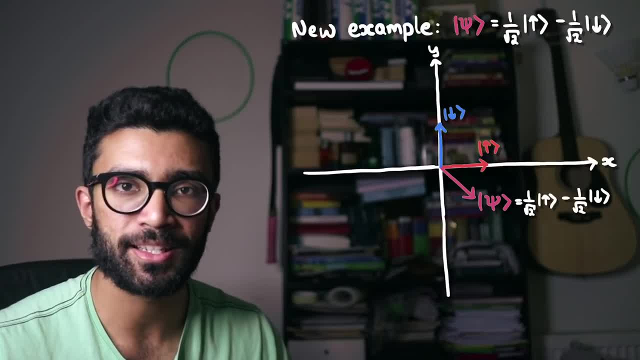 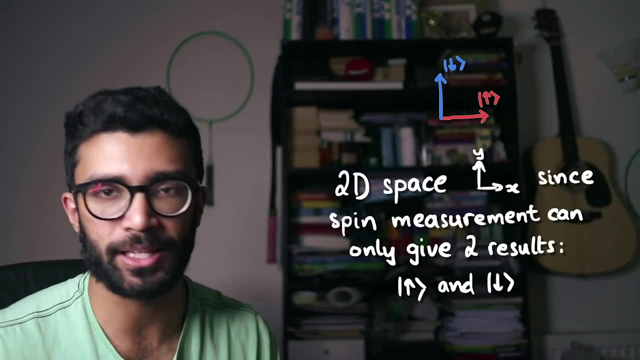 measurement result And because of this, any system that's in a superposition of these quantum states can be described by a single vector in this abstract space. In this case we've just thought of a two-dimensional space, because we only had spin up and spin down as the possible measurement. 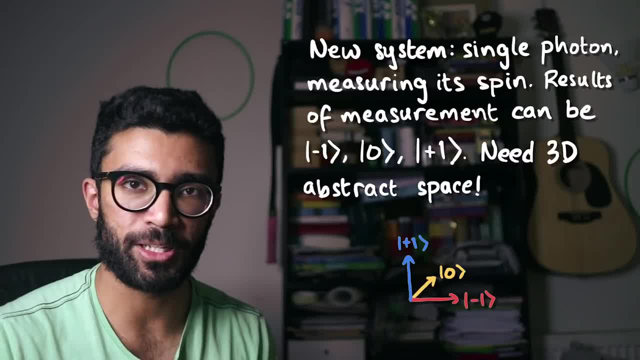 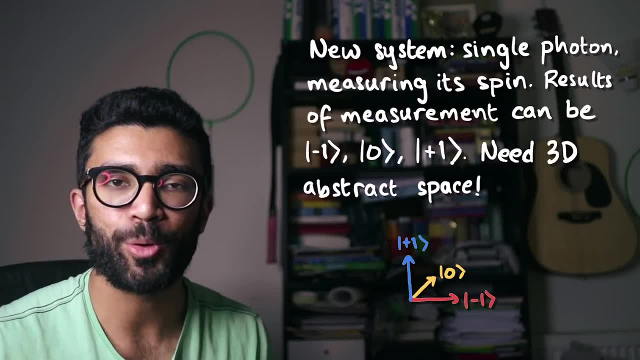 results. But there could be other systems where we had three possible measurement results which would be three-dimensional, and we'd have to represent our quantum system as a vector in this three-dimensional space. Equally, we might have a measurement where there are 10 different possible. 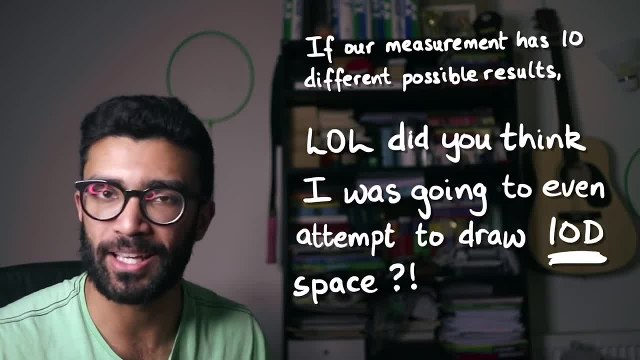 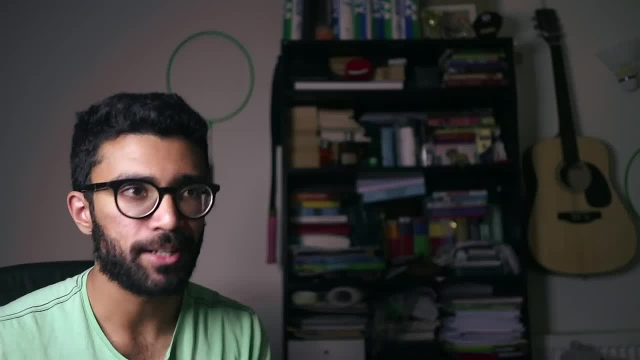 results. In this case we have to have a 10-dimensional vector space. Yeah, slightly difficult to draw but fairly simple to think about. Not necessarily imagine, because we can't visualize it, but we can just apply the same rules and imagine that there's going to be a 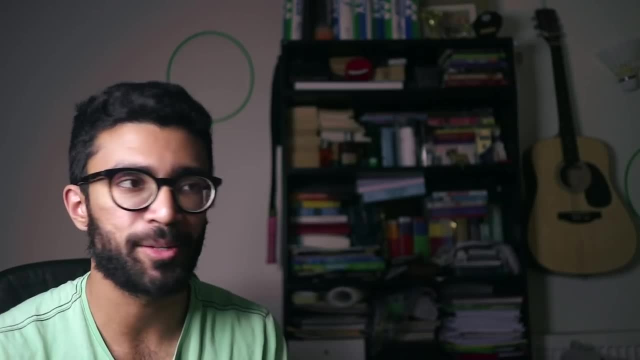 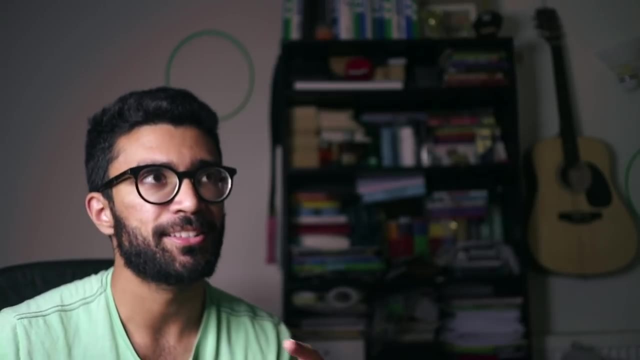 10 different, mutually orthogonal directions. So I hope you can start to see why this vector, representation of quantum states, becomes quite useful very quickly. And with all of that being said, I feel like I've talked about a lot. There's a lot of stuff that I haven't gone into detail. 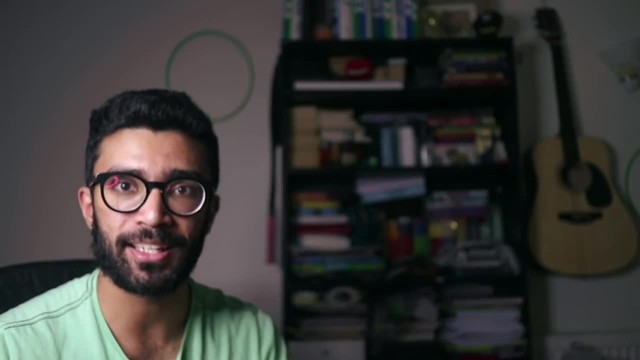 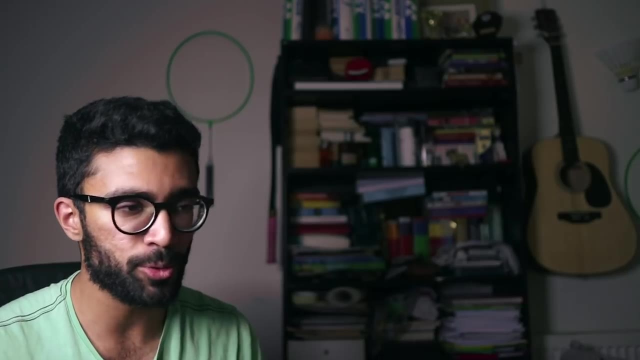 about, because there's a lot of mathematical intricacy that we need to understand in order to be able to even start comprehending some of this stuff, And essentially, what I wanted to do was to give you a flavor of how quantum physicists use mathematical notation to represent quantum. 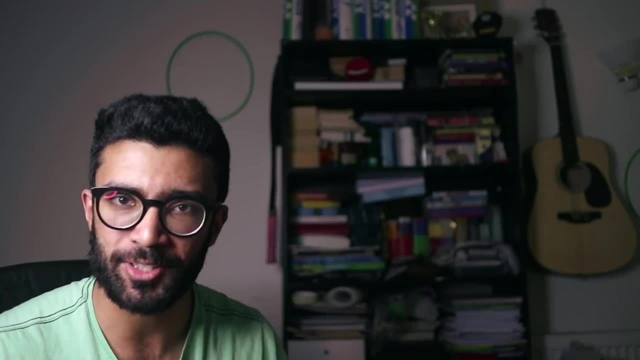 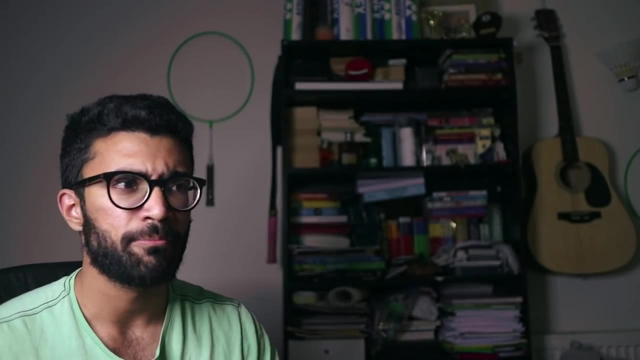 states. So I hope that this video has been helpful in some way in sort of shedding some light on that kind of aspect. I certainly know when I was younger, before I started studying physics at university, this whole field of quantum physics was very mysterious to me. There was not a lot that I knew. 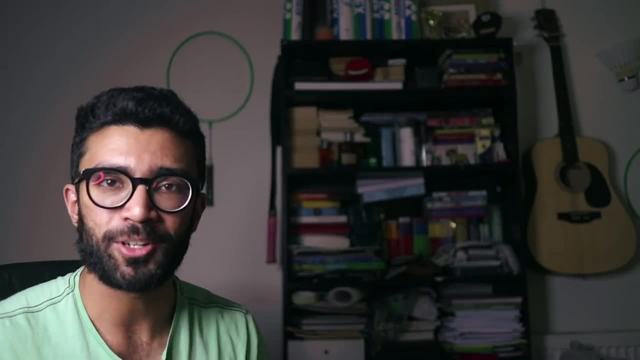 about it, apart from the fact that there are lots of weird results and weird ideas. So I wanted to make a video that would have been useful to me as a 16 year old in just understanding the kind of stuff that quantum physicists talk about and think about and the kind of mathematics they use to. 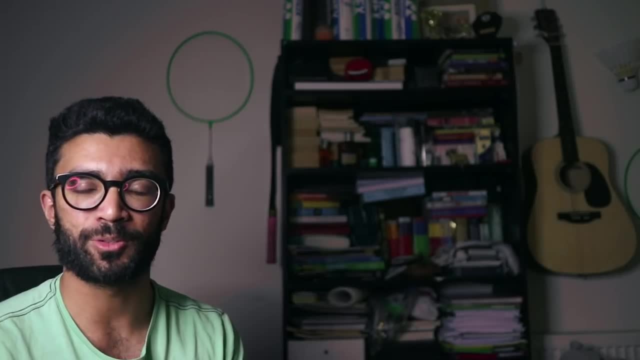 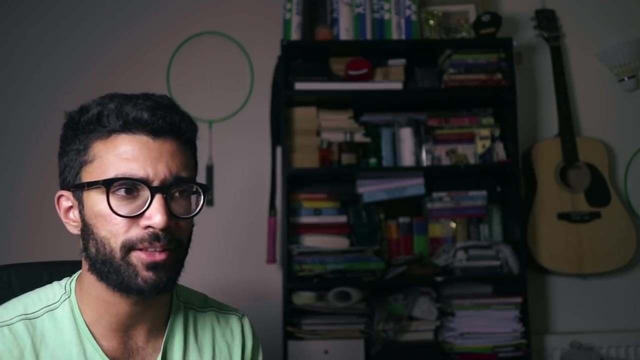 represent anything that they're studying. I hope that you found this useful as well, And I realized that there's a lot of stuff, like I said, that I haven't gone into detail about. So if you've got any questions, leave them down below And if there's anything that I haven't explained clearly, 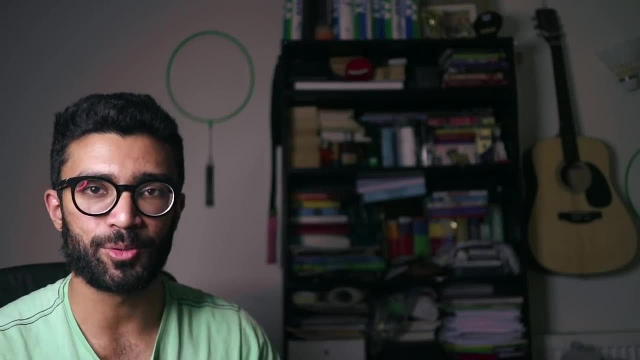 enough, then let me know in the comments down below as well. Additionally, if I've made any mistakes, then let me know in the comments down below as well. I'd like to put up a comment correcting that so that you guys don't leave with incorrect information. And I just wanted to say 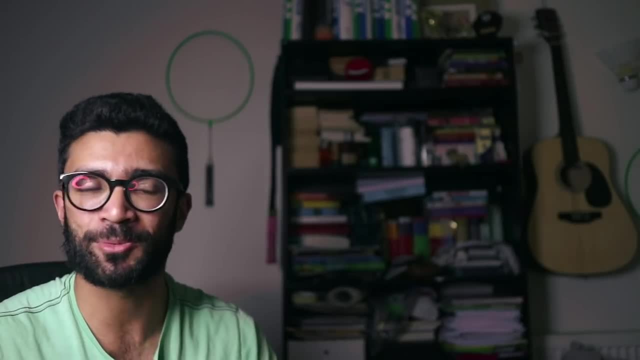 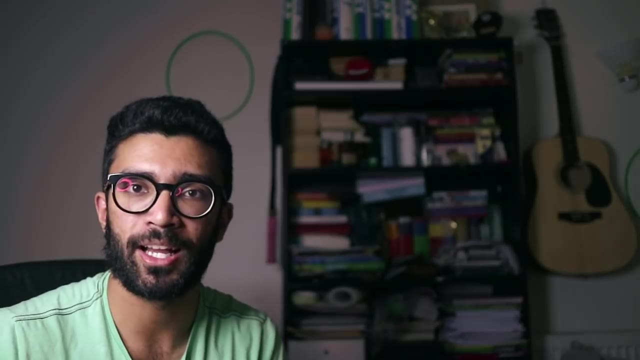 thank you to those of you who have left me nice comments on previous videos, And if you're going to leave me a nice comment on this video as well, thank you very much, But also those of you that give me constructive criticism. You know I'm trying to make these videos a bit better. I do. 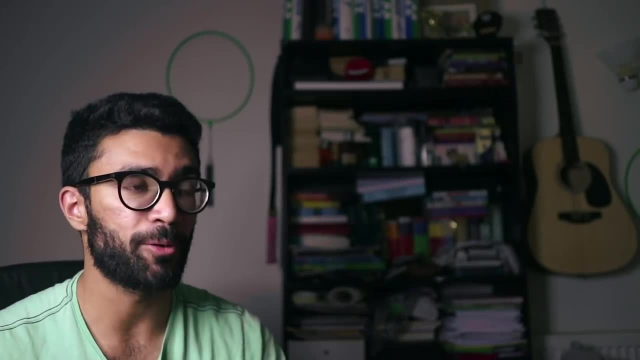 this in my spare time. This is not my full time job by any means. I just want to improve at making these videos. Hopefully they're enjoyable, Hopefully they're interesting And I hope that they're informative. With all of that being said, thank you so much for watching and I'll see you. 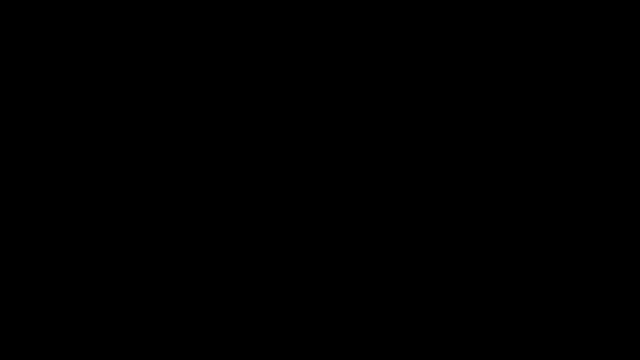